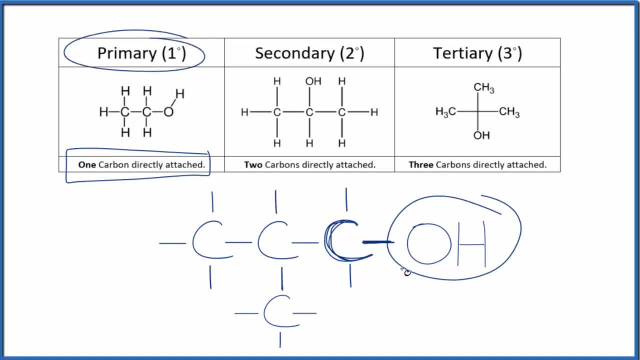 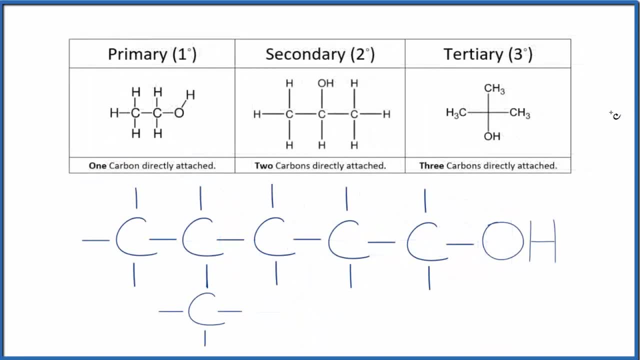 primary alcohol. So this is a primary alcohol. Note these lines right here. They go to hydrogen atoms, so we really kind of ignore them. Let's try another. So take a look at this one. Is it primary, secondary or tertiary alcohol? 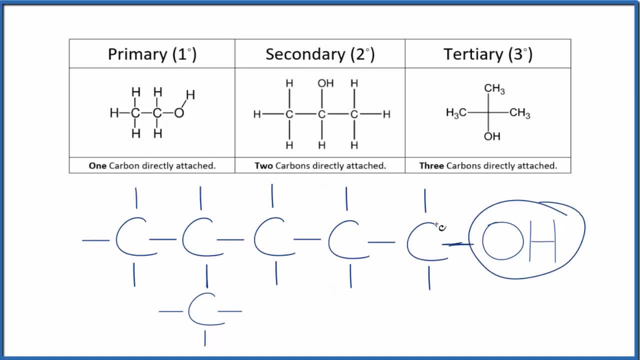 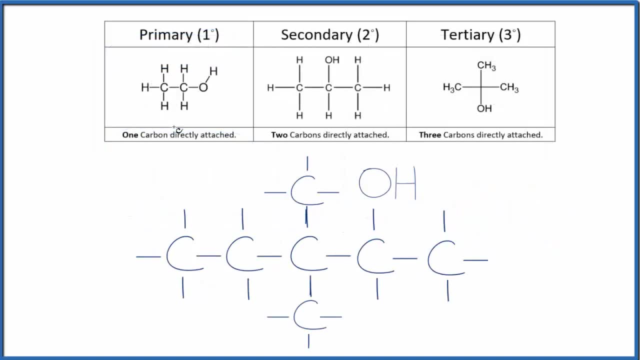 We find the OH group here. It's attached to just one carbon. That means it's a primary alcohol. So pause and give this one a try. So we find the OH. That's what makes this an alcohol. And we see the alcohol is bonded to. 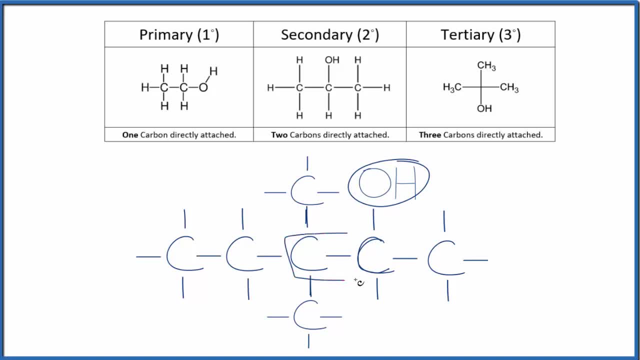 this carbon right here. This carbon right here has two bonds. It's two carbons directly attached to it. If there are two, that is a secondary alcohol. So we find the OH group here. It's attached to just one carbon. That means it's a primary alcohol. 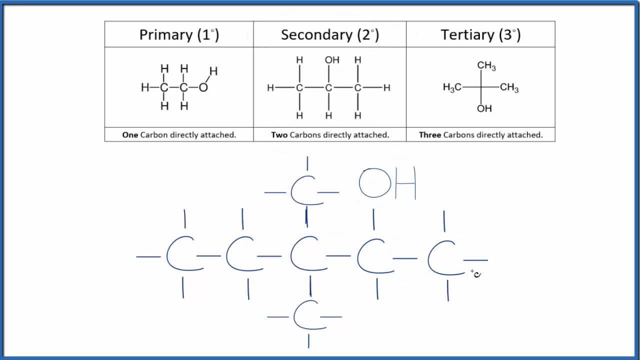 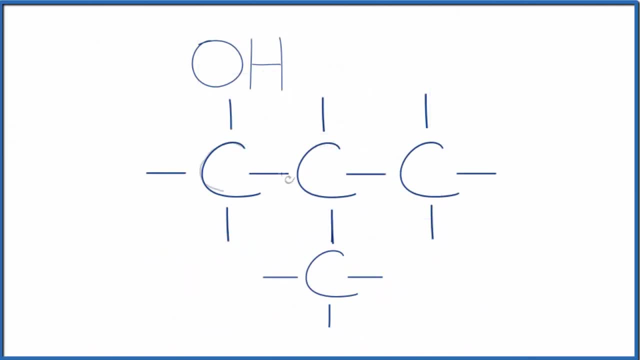 So, for this example, we have a secondary alcohol. How about this one? Pause and try this one without the table. So we find the OH group and here's the carbon that it's bonded to, right here. So this carbon, it's only bonded directly to one other carbon. That makes it- you guessed it- a primary. 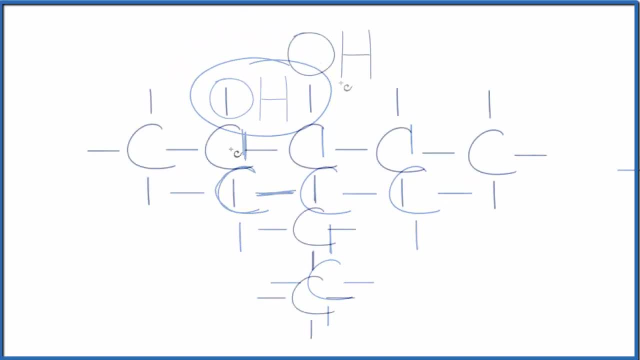 alcohol. How about this one? Here's the OH group. That's a primary alcohol And we see the OH group. it's bonded to this carbon right here And we can see this carbon. right here We have one, two, three carbons directly attached to the carbon that's attached to the OH group. That makes this a 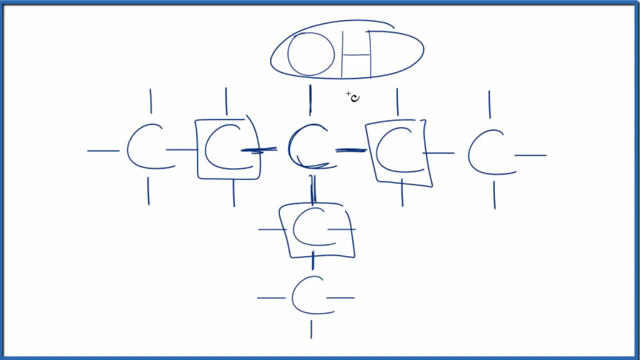 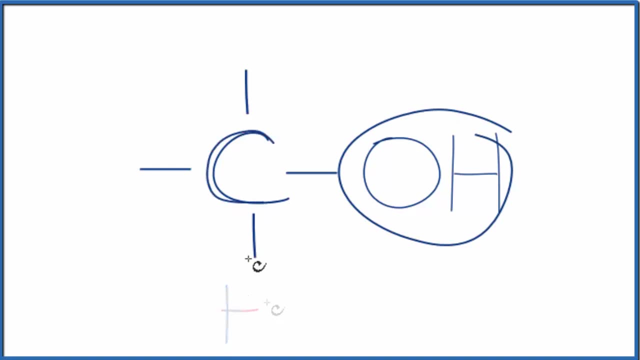 tertiary alcohol. This next one's a bit of a trick. This is methanol. So we find the OH group and here's the carbon. But this carbon's only bonded to hydrogens. They're not written, but they're there. So 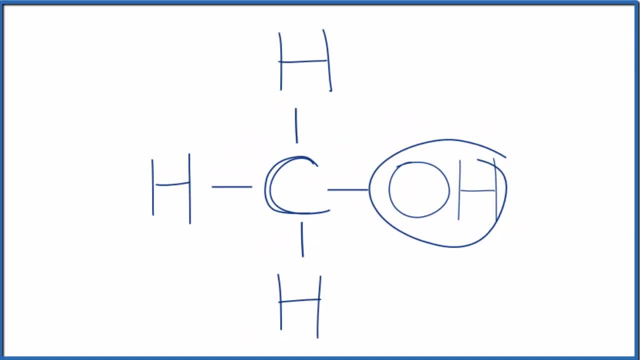 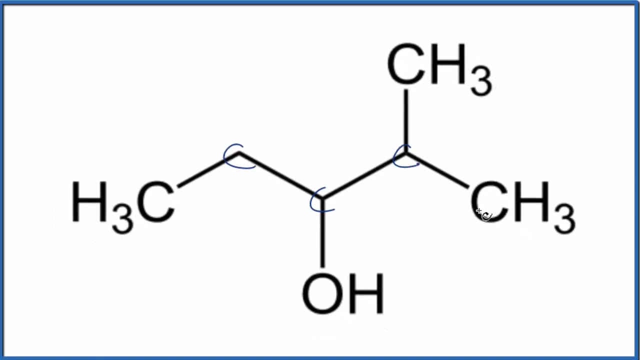 methanol is a bit of an exception. We call this a primary alcohol, even though the carbon's not bonded to any other carbons. Just the way we do it. Here's one that's written a little differently, in a more skeletal format. The trick: here: we have carbons at these junctures, So is this a primary? 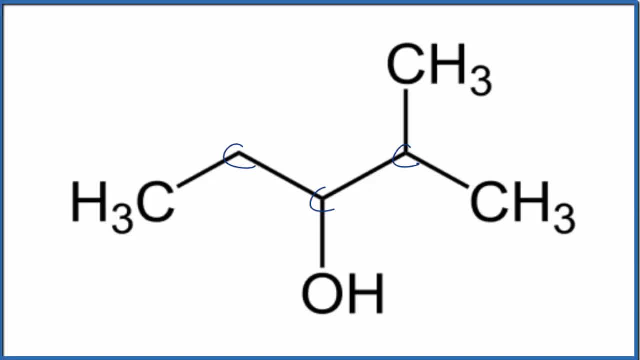 secondary or tertiary alcohol. If we find the OH group, we find the OH group. And here's the OH group. If we find the OH group, it's bonded to this carbon right here, which is bonded to one, two other carbons.